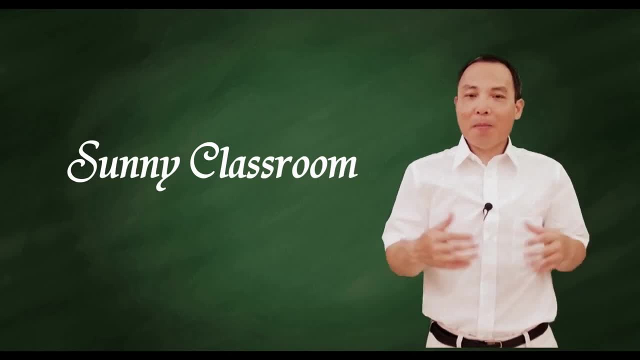 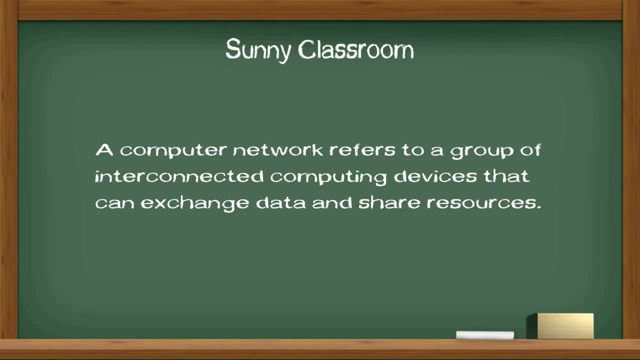 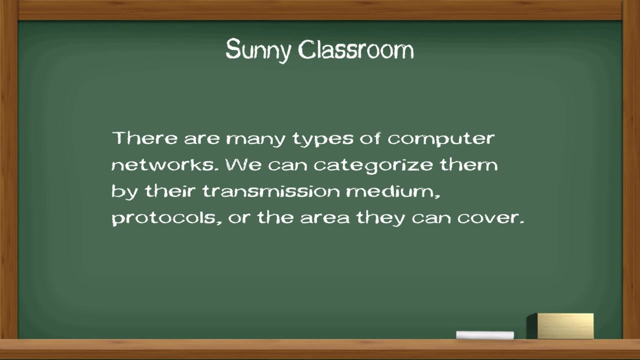 Hello, and this is Sunny, Welcome back. A computer network refers to a group of interconnected computing devices that can exchange data and share resources. There are many types of computer networks, and we can categorize them by their transmission media, protocols or the area they can cover. 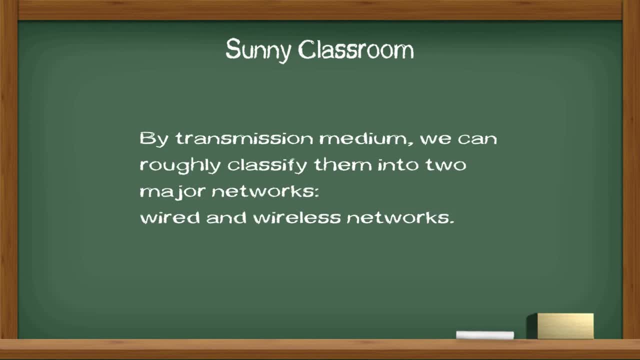 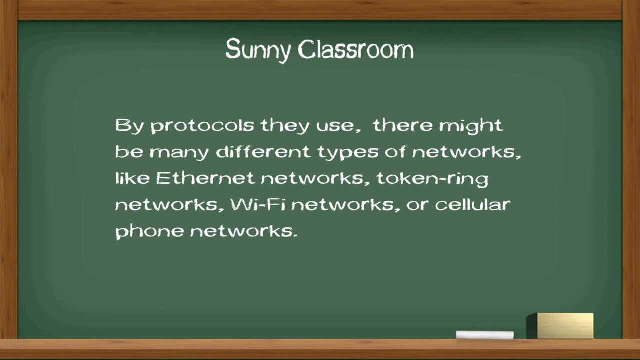 By transmission media, for example, we can roughly classify them into two major networks: wired and wireless networks. By protocols they use, there might be many different types of networks, like Ethernet networks, token-ray networks, Wi-Fi or cellular phone networks. 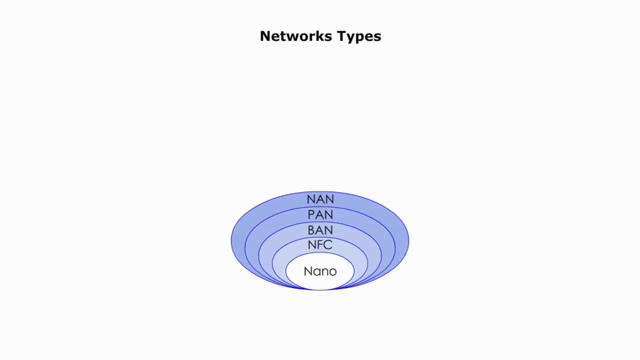 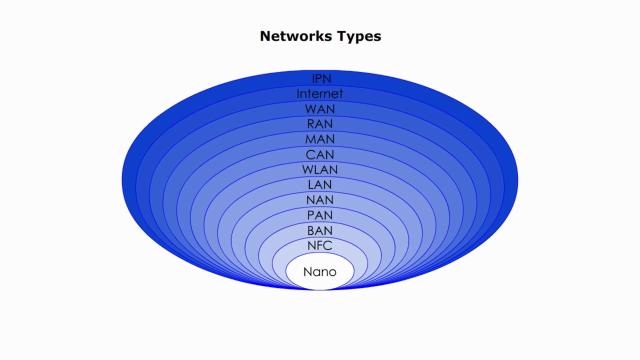 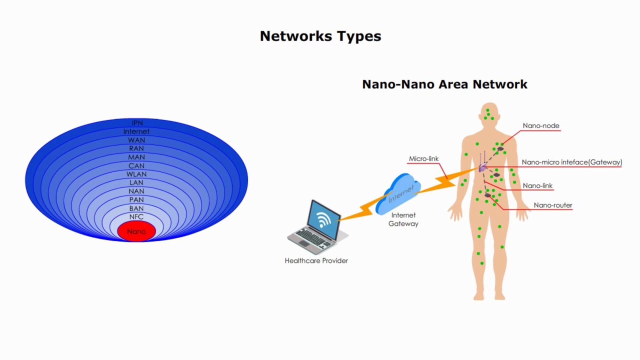 Today I will briefly talk about 13 networks. There are many different types of computer networks by spatial scope, the area they can cover. Let's start with nano area network. Nano, a set of interconnected super-tiny nanomachines, or nanorobots. 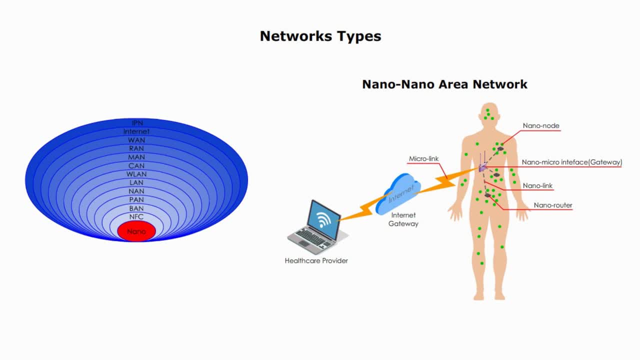 Nano is a unit prefix meaning one billionth. For example, a nanometer is one billionth of a meter. It is a super-tiny nanometer. It is a super-tiny unit used in the micro world. Nano can be used in many areas, such as weather, military industries and healthcare. 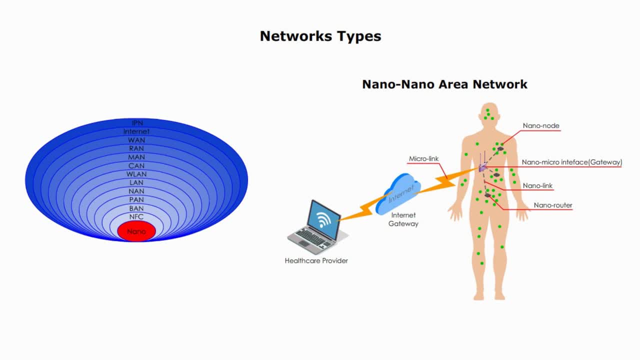 It can be lifesaver for millions of patients. These nanomachines could navigate through our bodies for diagnosis and treatment. For example, they can travel in blood vessels to clear blood clots or cure cancer cells. In this area, nano is largely in the research and development phase. 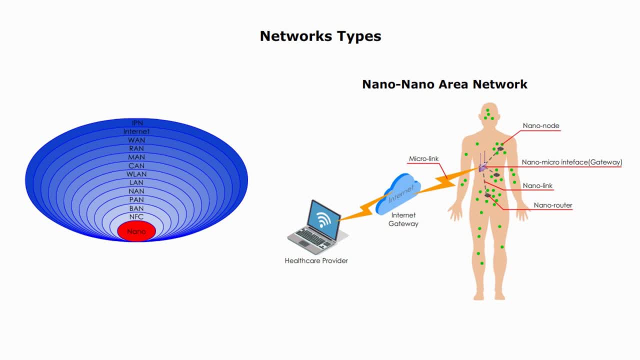 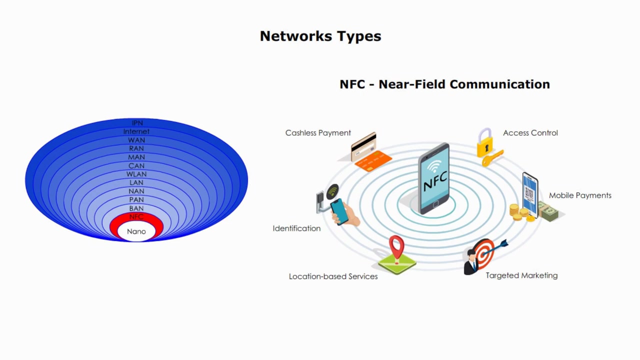 In the near future, nano can change our life on many levels. NFC- near field communication. Near field communication is wireless technology that enables two devices to communicate within the brain. It can communicate within very short range, like one to two inches. Near field communication is used for many applications such as cashless payment or cell phone payment access badges, identity tokens, smart cards or many more. 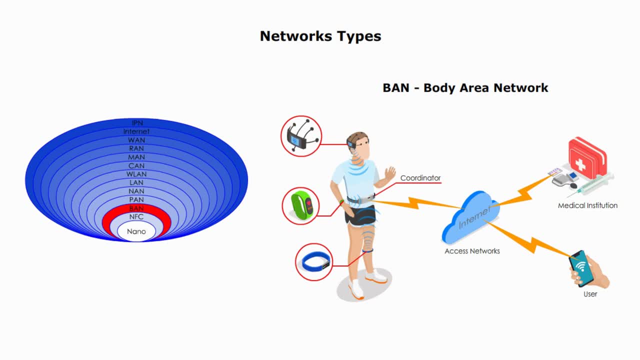 BAN, a body area network. BAN also refers to body sensor network. These sensors are in or on our human body, Such as blood pressure sensors, ECG sensors, body temperature sensors, insulin pumps, motion sensors or others to monitor our body's conditions. 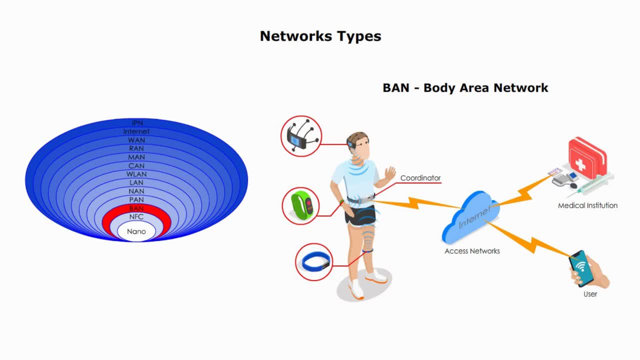 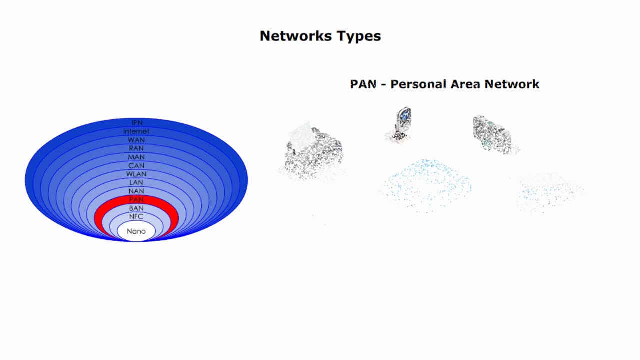 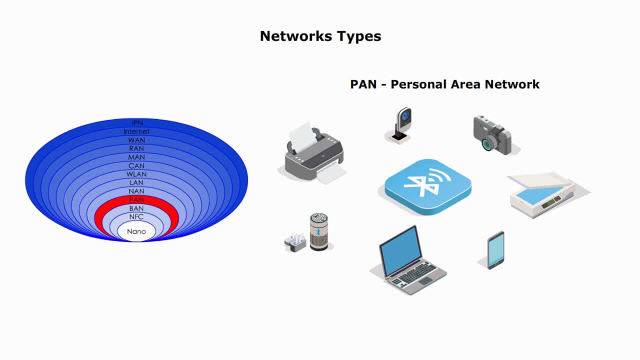 A BAN provides data transmission among devices such as computers, smart phones, tablets and PDAs. A BAN may be wired or wireless, utilizing wireless technologies such as wireless media. In this context, this system has gameplay potential With the convenient setup to compare input�� 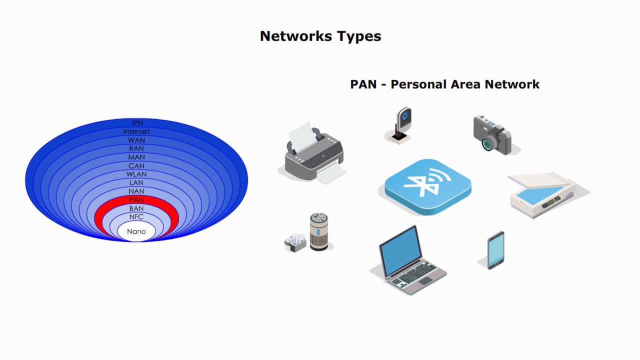 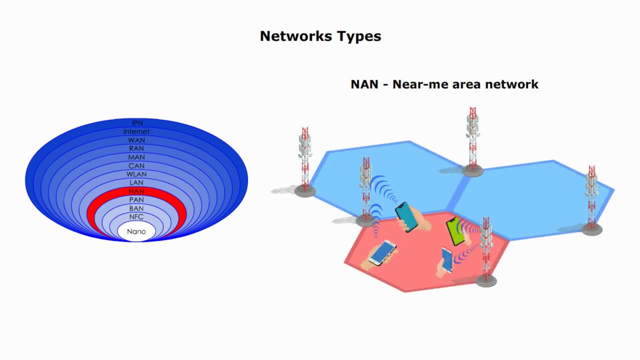 technologies such as wireless, USB, Bluetooth or ZigBee, Near Me Air Network. Nair applications focus on two-way communications among devices within a certain range. For example, I cannot go to see the movie, but I already bought the ticket At the entrance of the movie theater. I can send a message to anyone near me, Like who wants my. 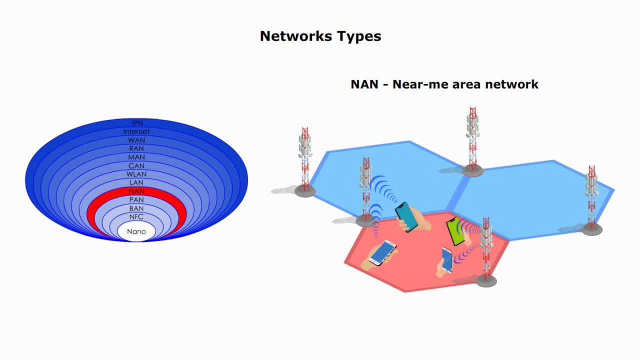 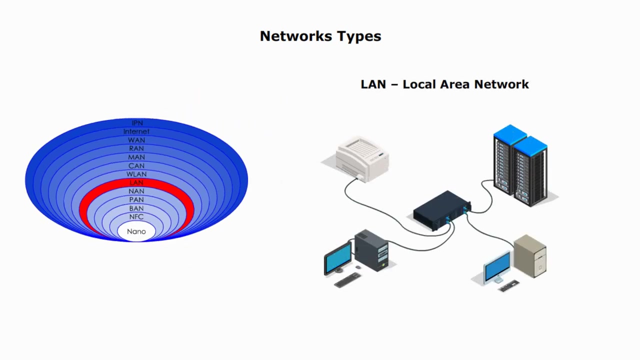 ticket is only half price. It's like a broadcasting over a short distance. The person who interested in my ticket can reply to me. He or she must be close by near me to get the message. Local Area Network: Most people are familiar with LAN. LAN is a group of computers connected at one location. 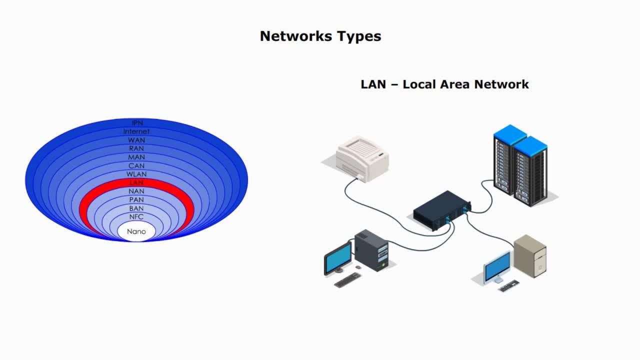 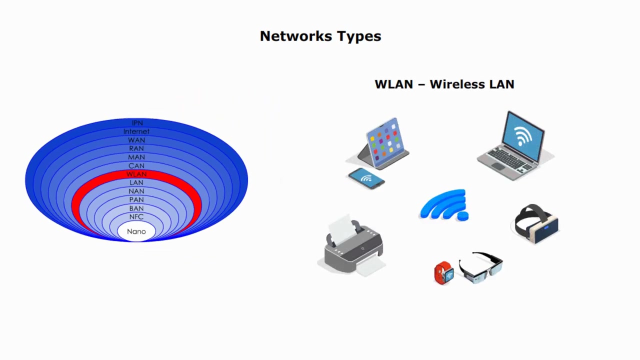 A LAN can be small or large, ranging from a small network at home to a network of thousands of users. Ethernet and Wi-Fi are the two most common technologies in use for local area networks. WLAN- Wireless Local Area Network- It's network based on radio transmissions rather than 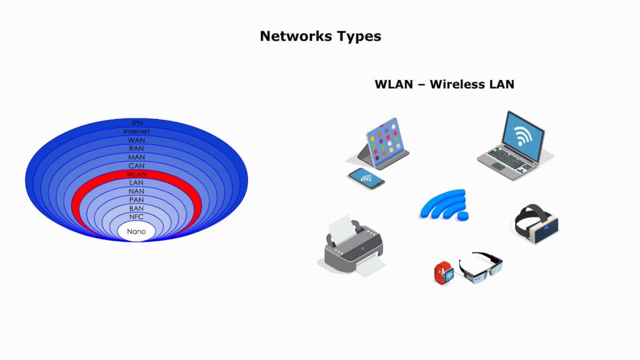 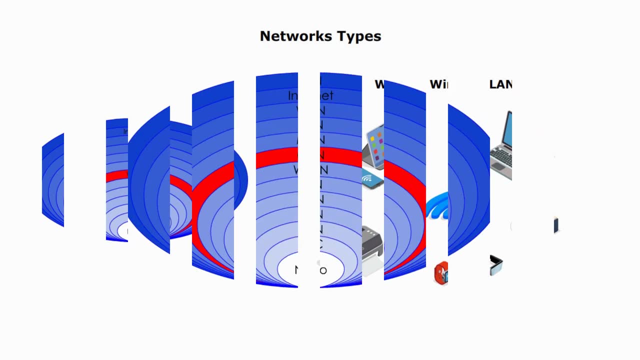 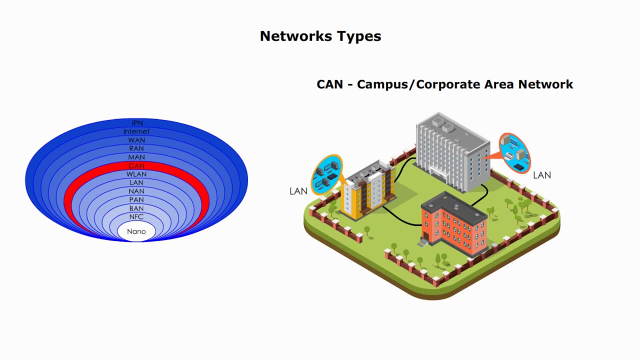 wired connections. A Wi-Fi network is a type of wireless LAN. Wireless LAN can be part of a local area network. CAN, Campus Area Network or Corporate Area Network is a computer network made up of an interconnection. local area networks lines within a limited geographical area. A CAM. 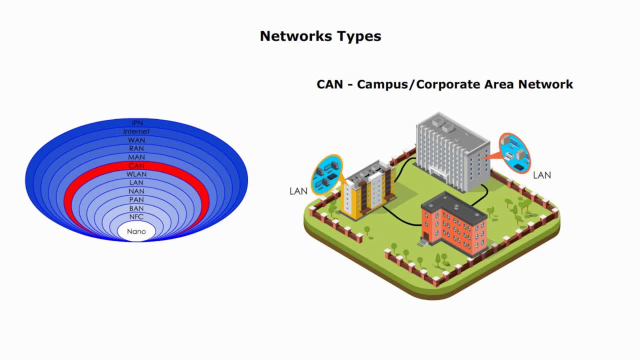 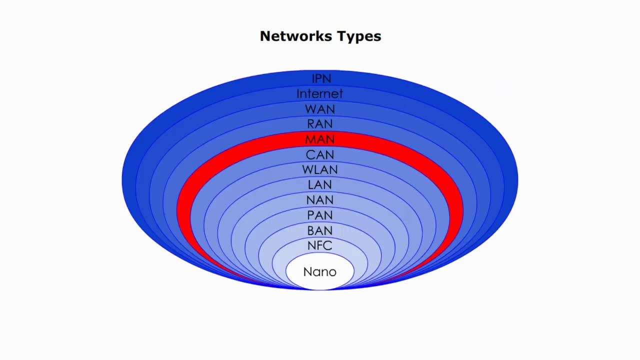 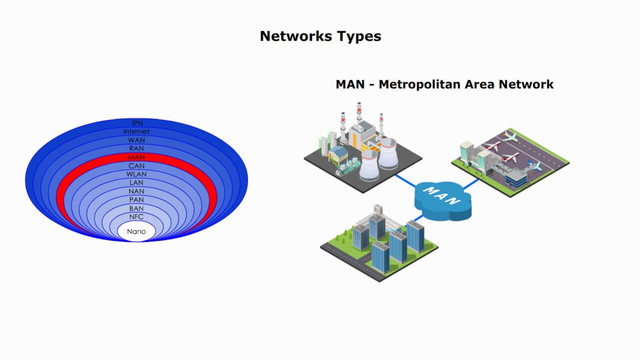 interconnects multiple lines within a educational or corporate campus. MET metropolitan area network: a computer network that connects computers within metropolitan area, which could be a single large city, multiple cities or towns, or any given large area with multiple buildings. RAINN Radio Access. 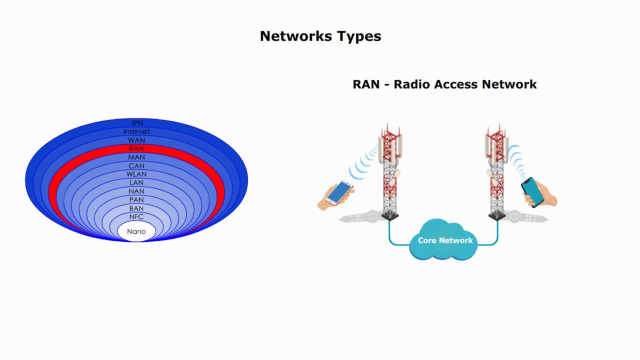 network is a part of cellular phone network that connects end users devices like mobile phones smartphones to call network. It is a part of the cellular phone network that connects users. devices like mobile phones smartphones to call network is a part of theơi. 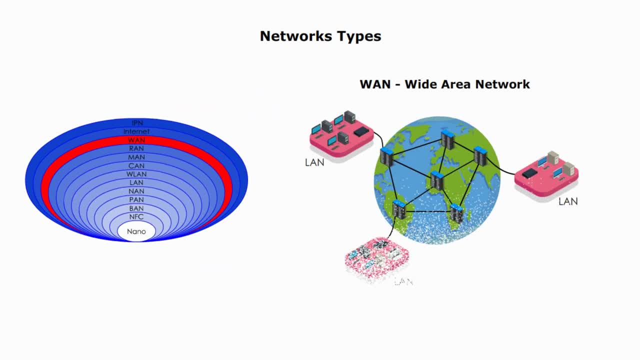 system One wide area network. A wide area network is a telecommunications network that extends over a large geographical area. In its simplest form, the wide area network is a collection of local area networks. lines One is essentially a network of networks We can consider the largest one in the world. 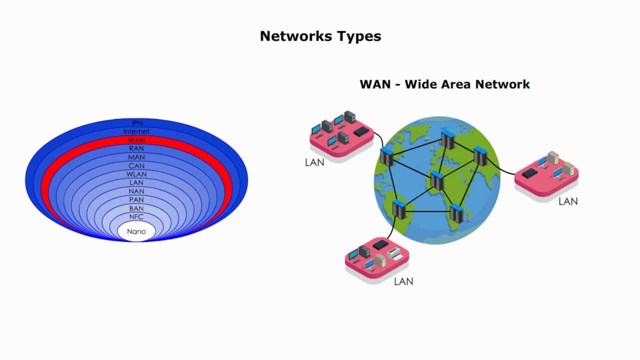 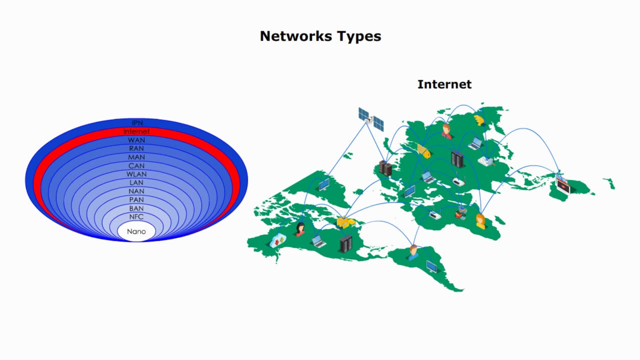 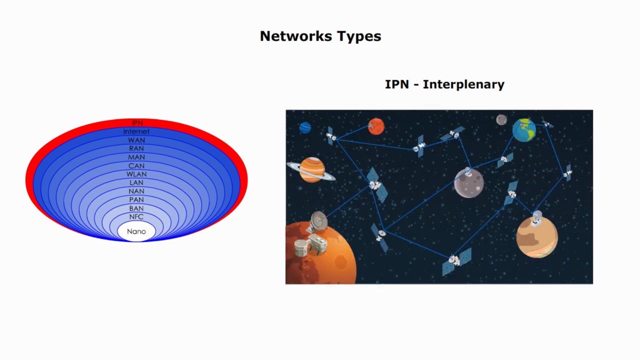 the Internet. The Internet is the global system of interconnected computer networks. It's a network of networks that consists of private and public networks of local to global scope, linked by the broad array of networking technologies, The last but not least, IPM, the Interplanetary Internet. 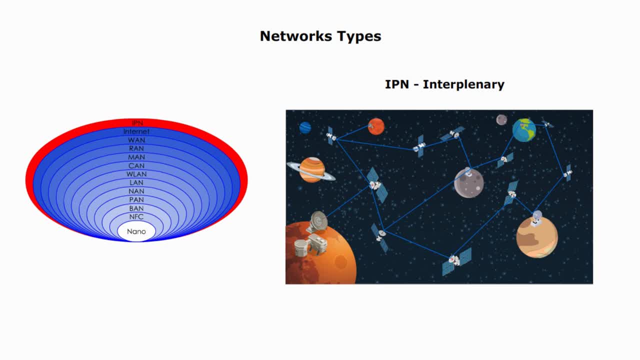 A computer network in space consisting of several network nodes that can communicate with each other. It's not a fiction, but a real thing coming soon, Very soon, with NASA's Deep Space Network. we can watch Netflix on Mars with NASA's Lunanet, and you can share your photos on Instagram from the moon. 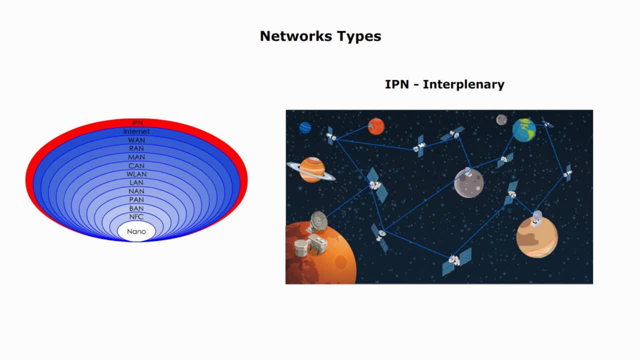 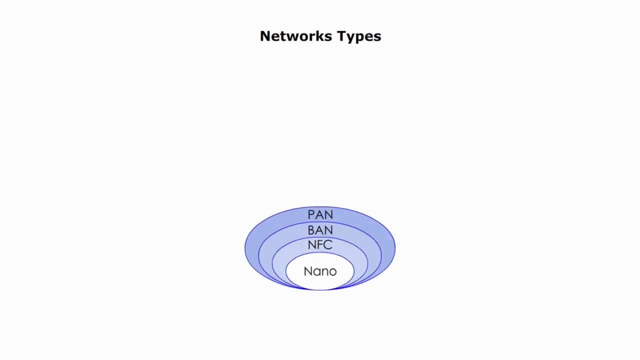 We don't know the future, but our future is very promising and exciting. It's not easy or clearly defined the boundary of these different types of networks. It's not easy or clearly defined the boundary of these different types of networks. It's not easy or clearly defined the boundary of these different types of networks. 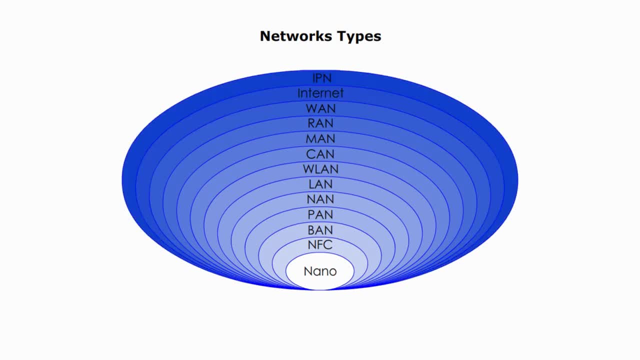 The area they cover can overlap and the technologies used in different networks might be the same. It's understandable if you feel confused a little bit. Categorizing computer networks is complex after all. Thank you very much and see you next time.